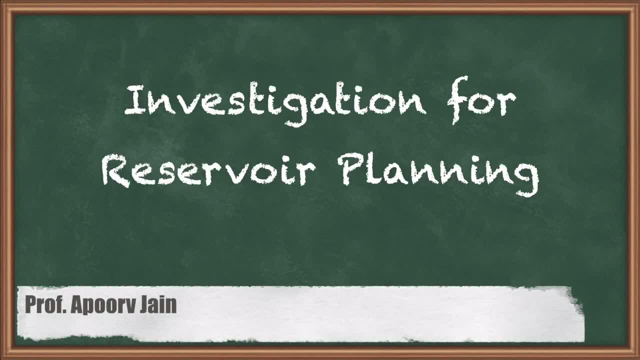 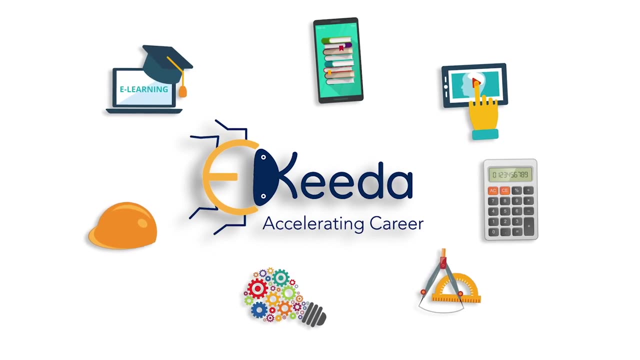 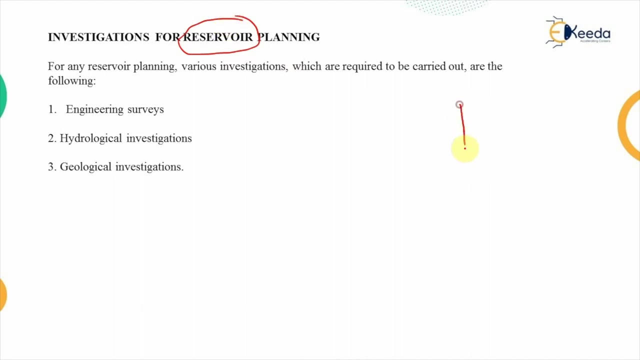 Hello everyone. in this video, we are going to study about the investigations which are carried out whenever we plan a reservoir. So let's start. So what is a reservoir? that we have already seen? So it is a barrier which is constructed across a river to store the water or for any other purpose that may be related to the level of water in the river. 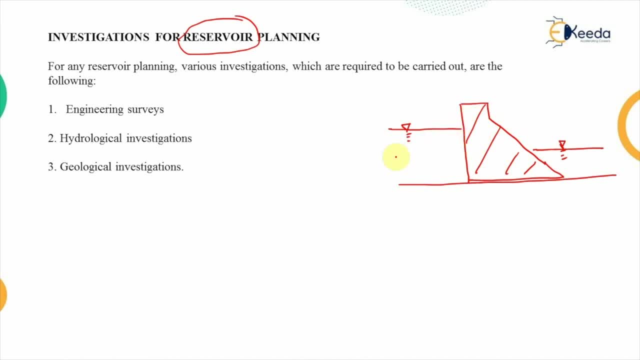 Now to plan this reservoir, which is storing the water or is avoiding the flood, we have to design this structure. So for any reservoir planning, various investigations are required to be carried out, And they are majorly classified in three categories. First one is that we need to carry out the extensive engineering surveys. 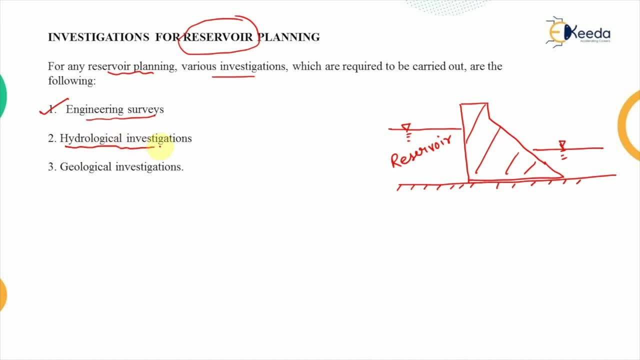 That is the first one. Second one is the hydrological investigations which are to be carried out. That is what is the majorly classified. Third one is the natural rainfall condition in the particular area where this reservoir is to be situated. What is the return period of a particular storm? 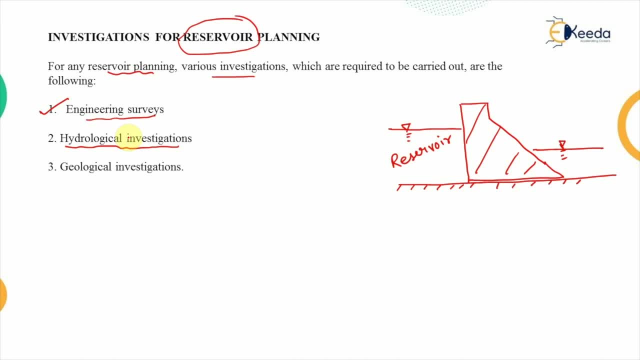 How many, or what is the capacity of the channel to carry the water. All of these is to be taken into account. And the third one is the geological investigation. That means what is the structure of the rock Or the earth crust beneath the reservoir? 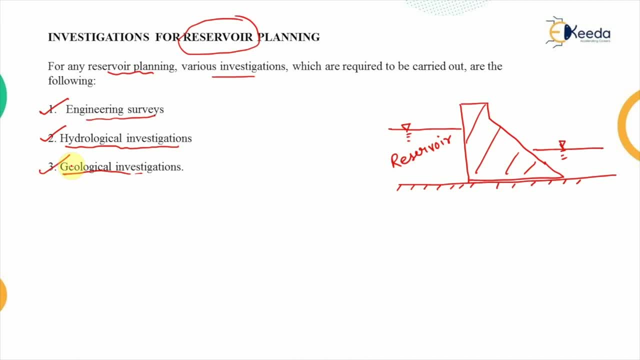 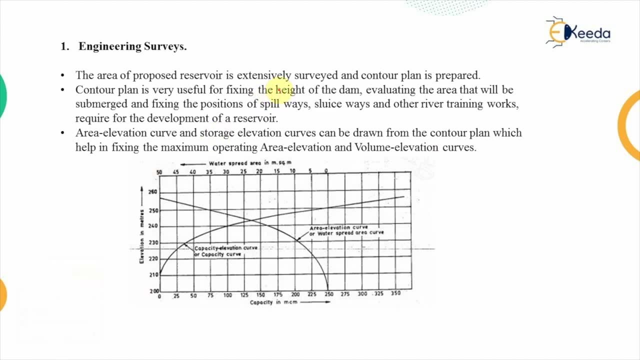 All of these factors are to be accounted. So first one is the engineering surveys. Now, when we talk about the engineering surveys- the area of the proposed reservoir that is extensively surveyed and corresponding to that, we prepare the contour plan. Now, what is this contour plan? 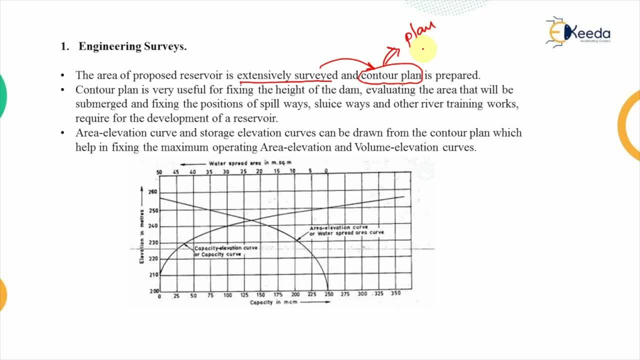 So this is a plan which is showing the lines joining points of equal elevation. It is a plan which is showing the lines joining the points of equal elevation, So the points which are at the same elevation from the mean sea level, they will be located or will be represented by a line. 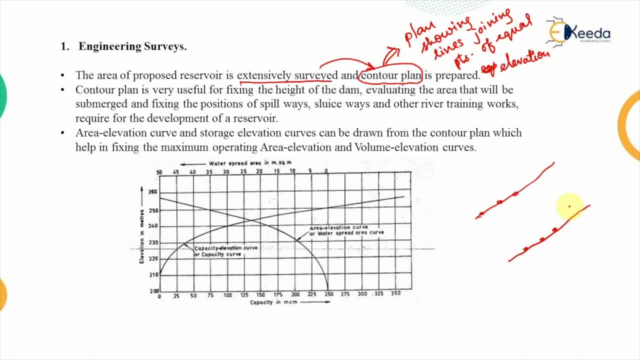 The other one, which are at the lower level. they will be connected by another line. So the difference between these two will tell us that from which line the flow will be taking place And towards which line the water will be going. That we will get to know with the help of this contour plan. 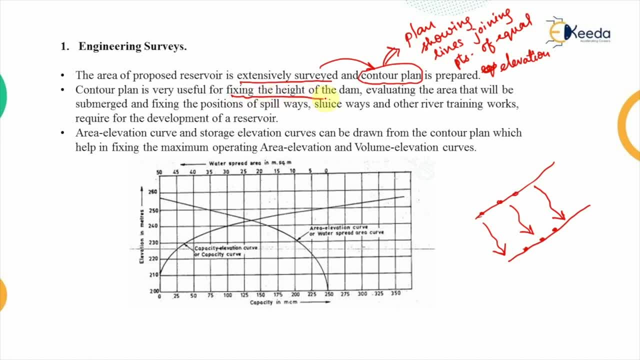 Now, this contour plan is very useful for fixing the height of the dam, Because based upon that only, we will prepare the head difference And we will evaluate the area that will come under the effect of the flowing water And that will be submerged. 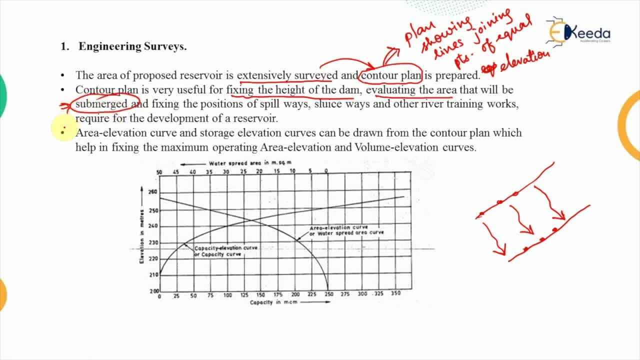 Because this is the major problem whenever we create any kind of reservoir. So we need to rehabilitate the people which are inhabiting in that area. We need to move them into a certain new position. So for that we need to correctly evaluate the area that will be submerged. 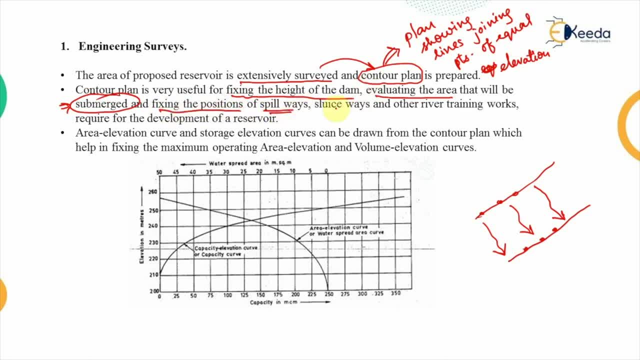 And fixing the position of the spillway or the sluiceways Or whatever river training work that we are providing in the development of a reservoir. Now, for this purpose, the area elevation curve and the storage elevation curve: they are drawn from the contour plan. 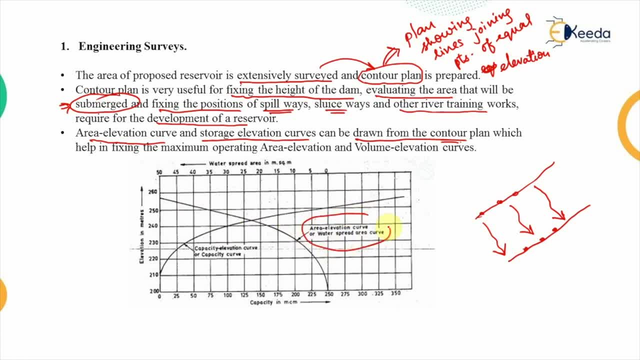 So, as you can see, this first curve is representing the area elevation curve. That means, with the increase in the elevation, As we are increasing the elevation, the water spread is also increasing Because if, let's say, we are storing the water at certain higher location, 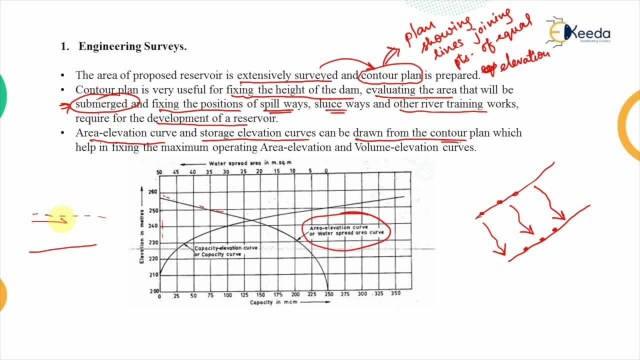 So the area which will be submerged if that is released that will be a higher area. But if we are storing the water on a flat terrain, That means at lower elevation the spread of the water will be very less. Similarly, the other curve is the capacity elevation curve. 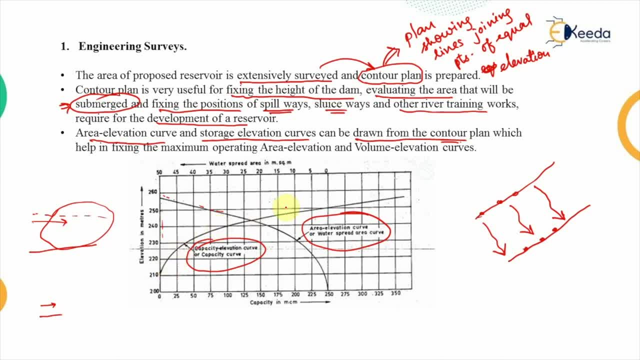 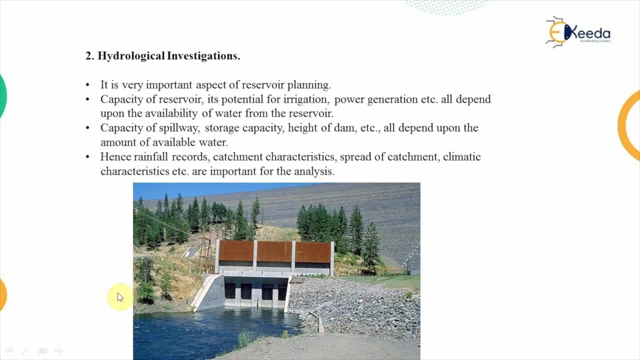 So as we are increasing the elevation, the capacity is also increasing. So both the curves are the increasing curves with the elevation. Next survey is regarding the hydrological investigation. Now, it is also a very important aspect, Because only the hydrological parameter tell us about the return period. 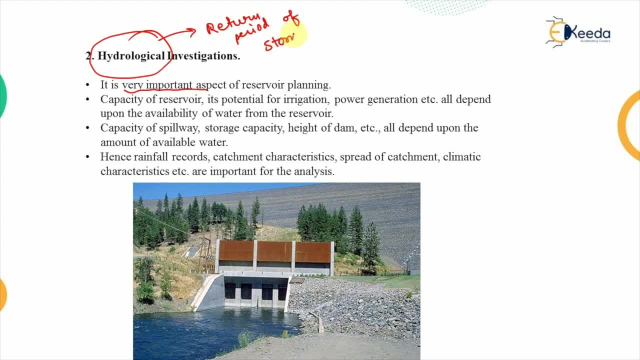 Tell us about the return period of the storm that we commonly call as the flood, So that after what duration the same flood of the same intensity or the magnitude will be returning to that particular area, And based upon the frequency of those floods we would like to design our structure. 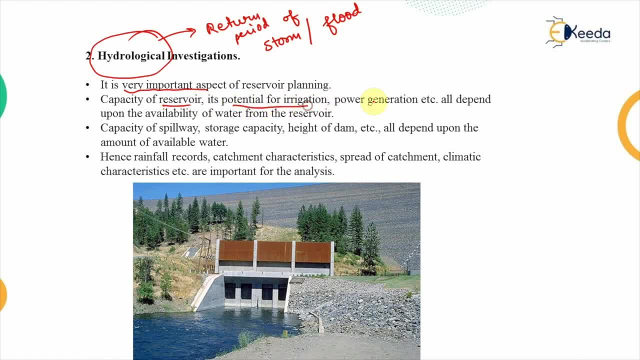 So the capacity of the reservoir, its potential for irrigation or power generation, All of it depends upon the availability of the water from the reservoir. Now, this water is available through the rainfall, and that rainfall is studied under the hydrological conditions. So that's why we need to carry out the suitable hydrological investigations for the reservoir. 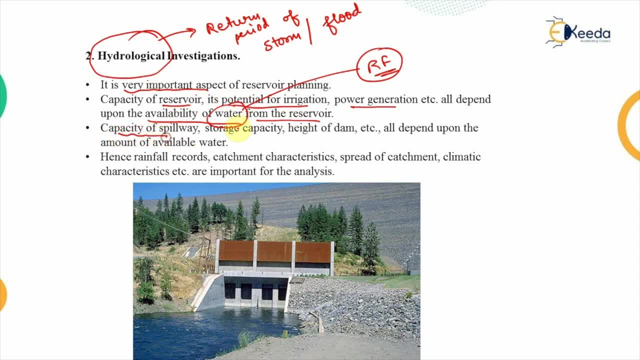 Now that in turn will affect the capacity of the spillway, The storage capacity of the reservoir and the height of the dam. All of this depend upon the amount of available water And for that, the rainfall records, the catchment characteristics, the spread of the catchment, the climatic characteristics. 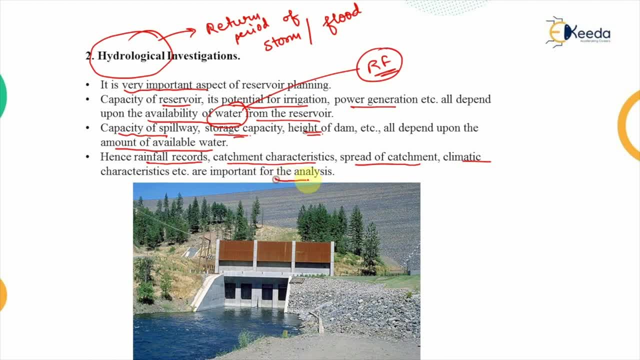 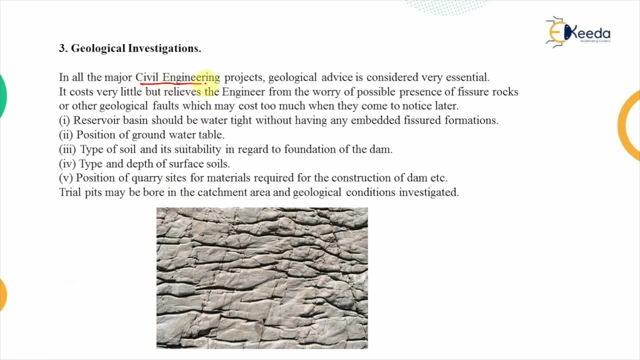 All of these are very important for the analysis of the reservoir hydrologically. And the last one in the investigations Is the geological investigation. Now, whenever we carry out any civil engineering project, Be it for the irrigation or for any type of construction, 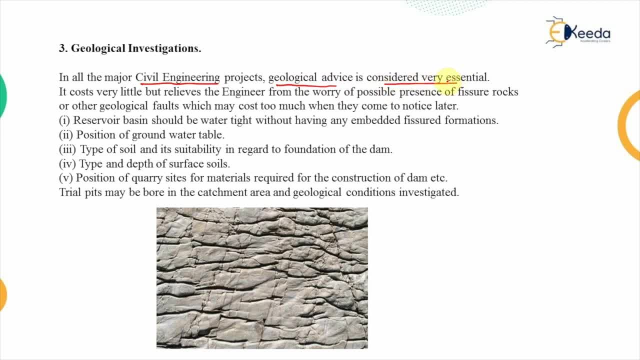 Geological advice is considered very essential Because initially it cost very little, But if there is a failure then it cost very dearly. So it relieves the engineer from the worry of the possible presence of the fissure rocks. Now this fissure rock is shown in the image. 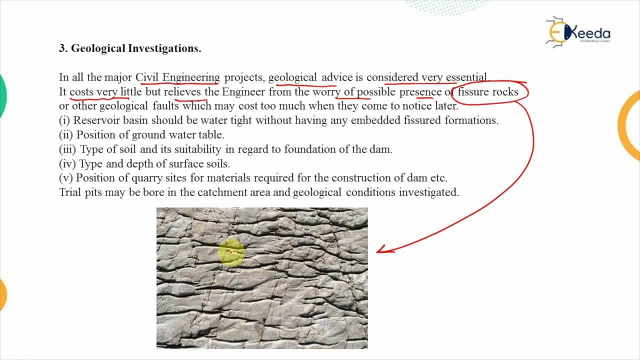 So these cracks which appear in the rocks, They are known as the fissures Or other geological faults. Now what will happen? As the earth is having certain plates on which the crust is resting. Now these plates, under the tectonic forces, they continuously move. 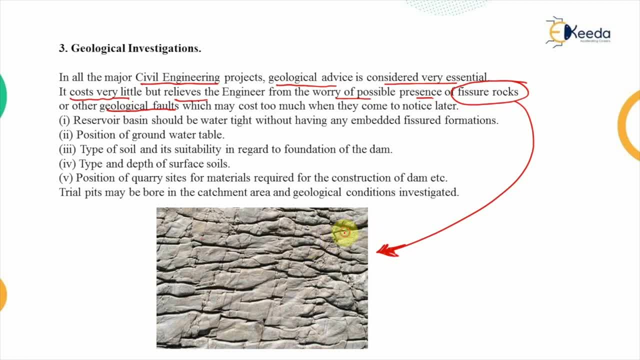 Now, if there is a friction between the two plates, There will be a movement which may cost too much If they are coming to the notice at the later stages, Because ultimately the structure will be doomed. So the reservoir basin, whatever we are constructing. 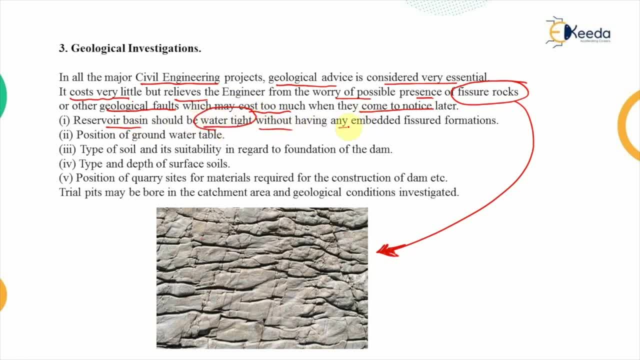 That should be water tight, Without any embedded fissured formations. That is the first thing that is kept in geological investigation. What is the position of the ground water table? If the ground water table is having the different elevation That it would be having certain uplift characteristics? 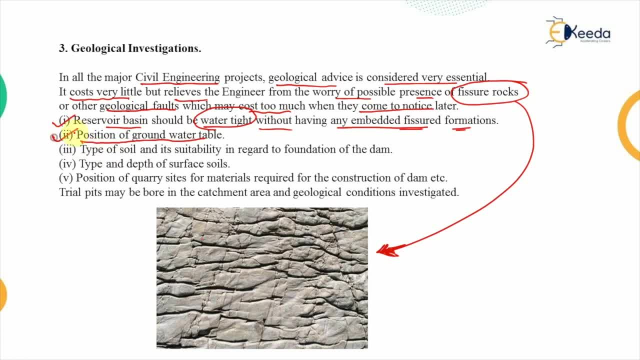 So that is why it is also an important criteria. Then, what is the type of soil? Whether it can sustain the weight of the dam, Whether it can be treated as the foundation of the dam or not, All of this is to be factored in. 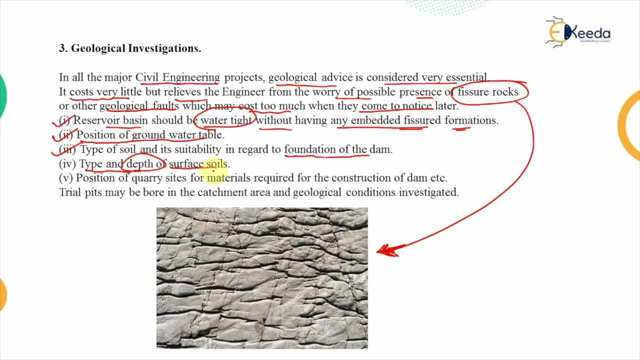 Then the type and the depth of the surface soil. It should not happen that the soil is only several centimeters deep, So the structure would not be supported on the rocks. It should have proper embedment And the position of the quarry sites for the materials.